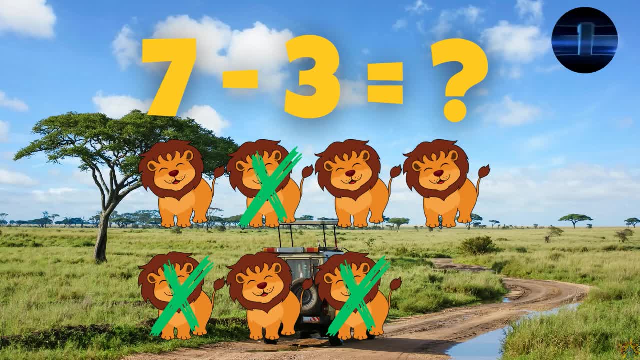 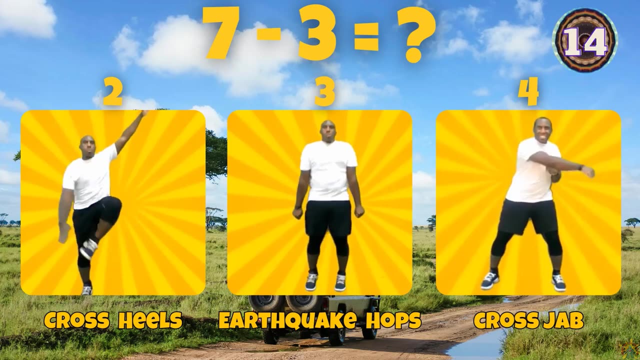 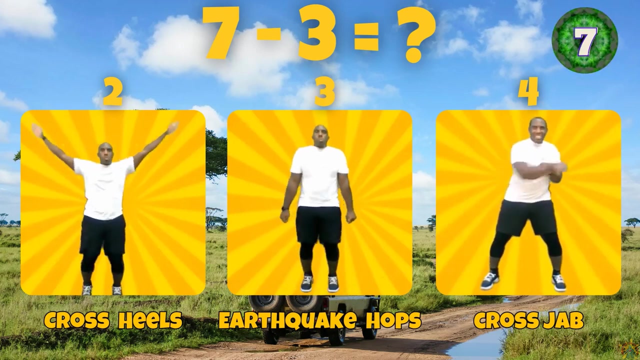 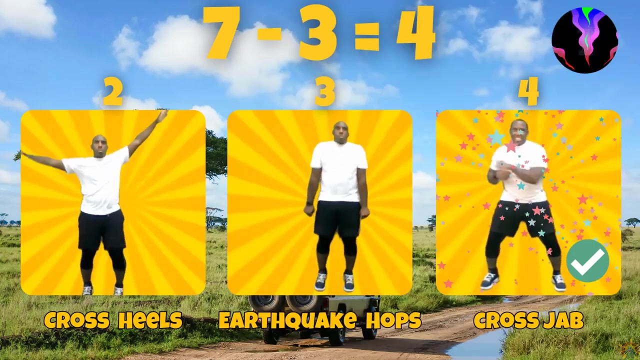 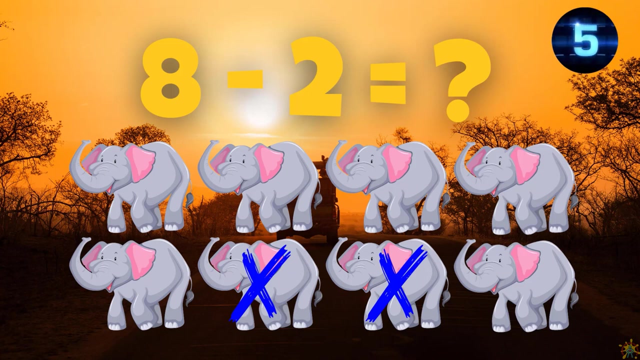 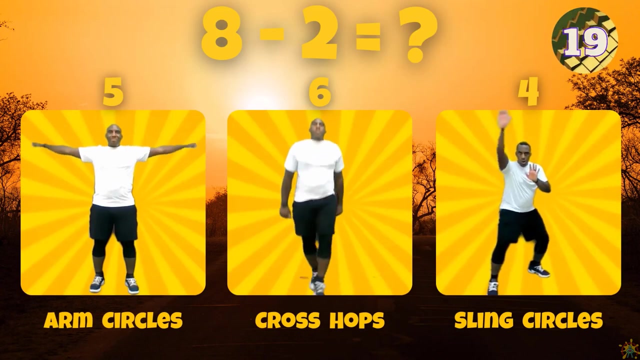 What is 7 minus 3?? Does 7 minus 3 equal 2, 3, or 4?? 7 minus 3 equals. 7 minus 3 equals 4.. What is 8 minus 2?? What is 8 minus 2?? 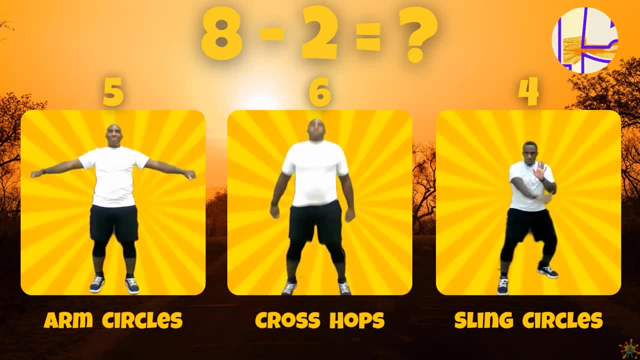 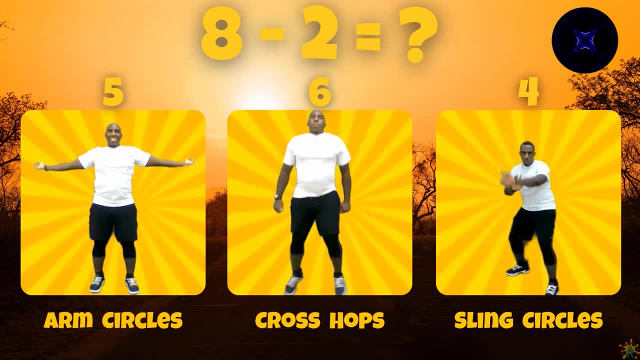 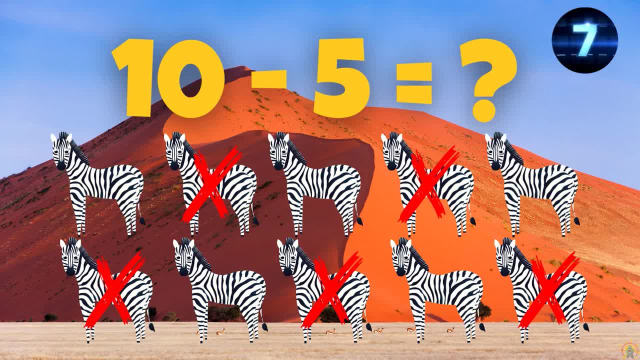 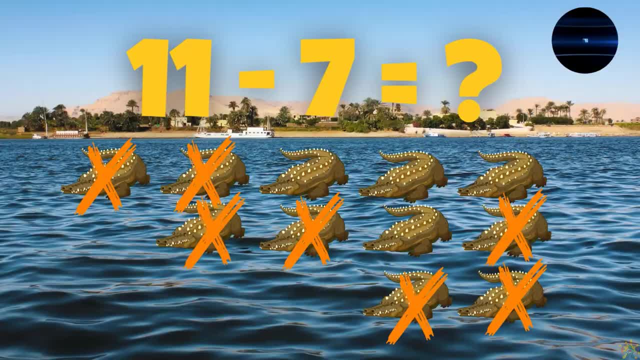 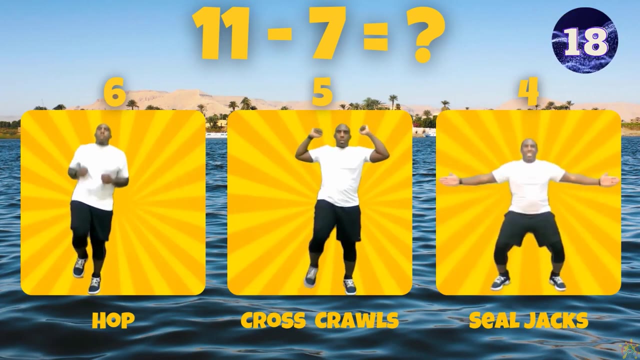